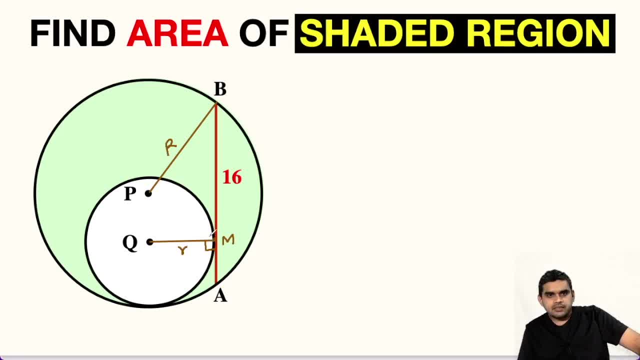 radius of this smaller circle, B. So this angle will be 90 degree and qM will be equal to small R, small i. Now the question comes why this will be 90 degree. So for that we have a theorem that if we have a circle, this is the center point of the circle and if this is any tangent, this is the. 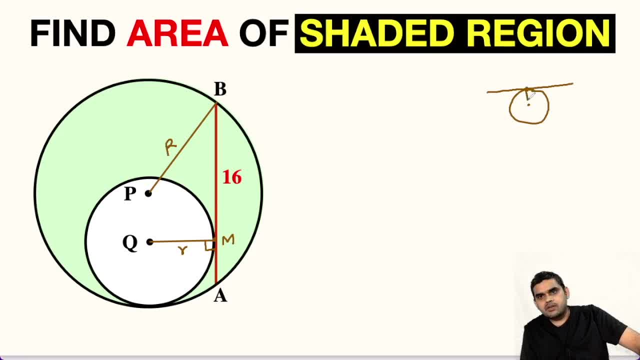 point of contact. So if you join the point of contact and the center of the circle, this angle formed is 90 degree. So here this will be 90 degree. Now, after assuming the radius of bigger circle as capital R and radius of smaller circle as small r, the area of shaded region can be written: 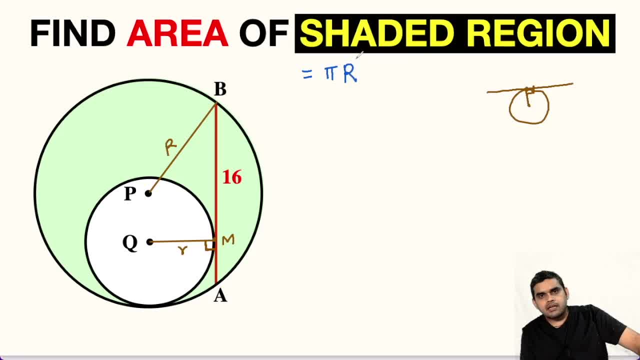 as pi times capital R square area of bigger circle minus pi times small r square area of this smaller circle. We can take pi common here, So this will be capital R square minus small r square. Pi is constant and if we are able to find this value of capital R square minus small r square, we can easily compute. 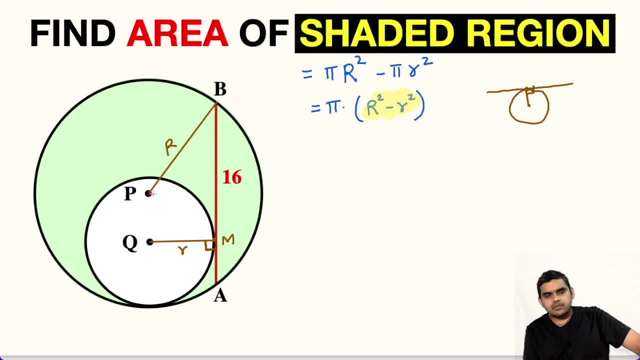 the area. Now let us do one construction here. From point P let us draw a line segment like this which is perpendicular to AB. So by construction this angle is 90 degree. We have another theorem that if we have a circle and this is the diameter of the circle, If this diameter of the circle 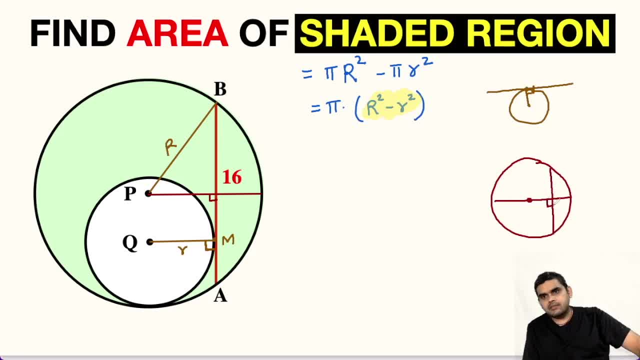 is perpendicular to any chord. say for example this: In our case AB is the chord, P is the center of the circle and by construction we are drawing this as perpendicular. So the theorem says that this length will be equal to this length. That means it will be perpendicular bisector. So if 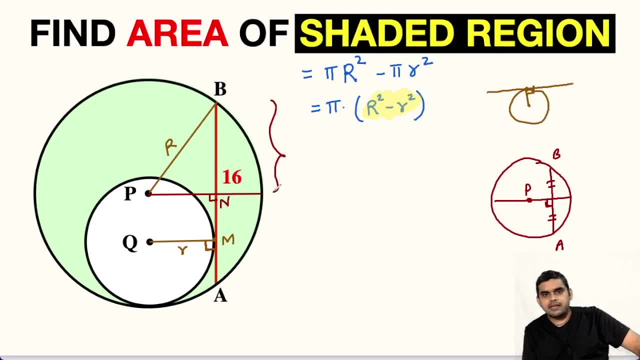 this point is N, then BN length will be equal to NA. So if the total length is 16, this will be 8 units And this will also be 8 units. Now, if we see by symmetry, the length of PN will be equal to this small r radius of this smaller circle. Let us write it here as small r.